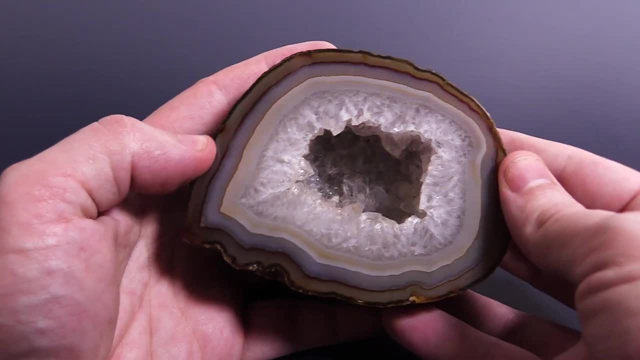 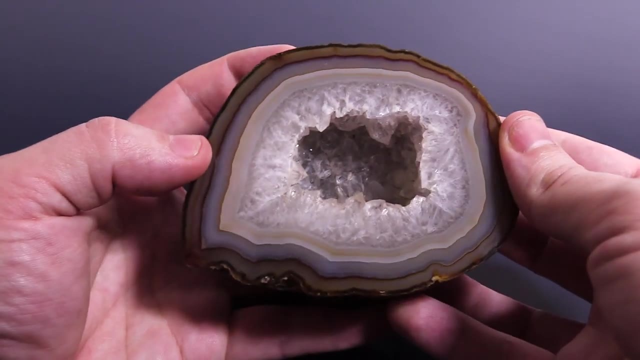 too much for at a gift shop. Agates are not fossils, because they are not the preserved body parts, excrement or impressions of an organism that lived in the distant past. but understanding how agates form helps us understand how permineralization works In the distant past. this agate was a cavity, a simple hole in a rock, a bubble that formed in lava as it grew. This agate was a cavity, a simple hole in a rock, a bubble that formed in lava as it grew. Rainwater slowly seeped through the lava rock and filled the hole, bringing microscopic minerals. 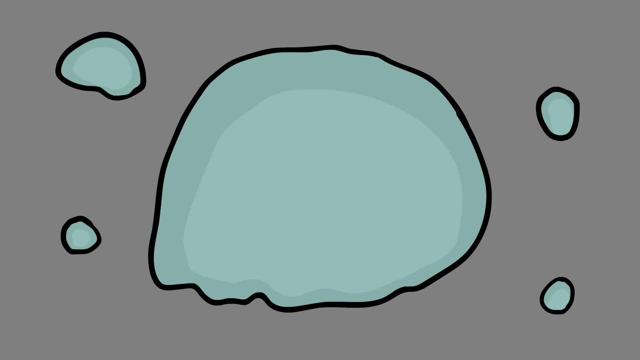 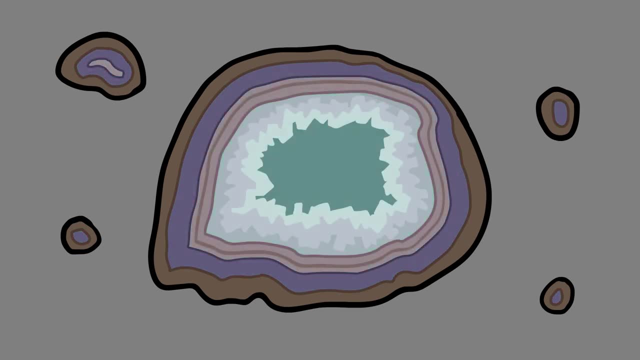 with it that were trapped as the water continued downward. When the mineral concentration was too high for the water to handle, the minerals crystallized, slowly, forming solid rings along the inside surface of the cavity. As you may have noticed, bones and shells also have. 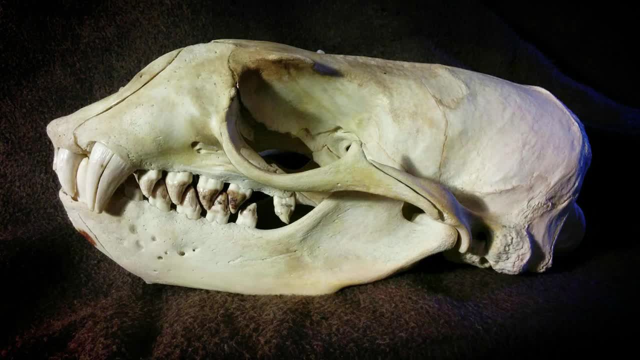 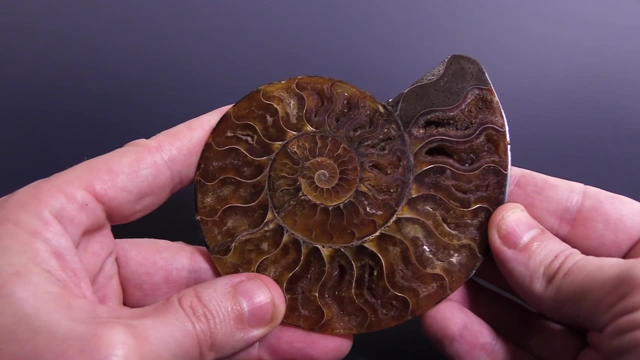 cavities: large cavities and microscopic cavities that can fill with mineral-rich water. In this ammonite fossil, you can see that some of the large cavities are still partly empty. This was also the case with my agate, but other chambers are completely full. They are completely. 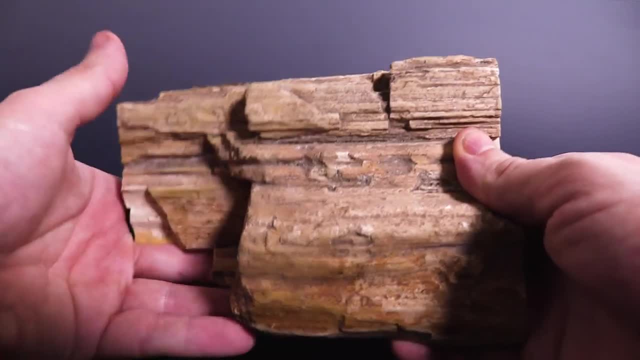 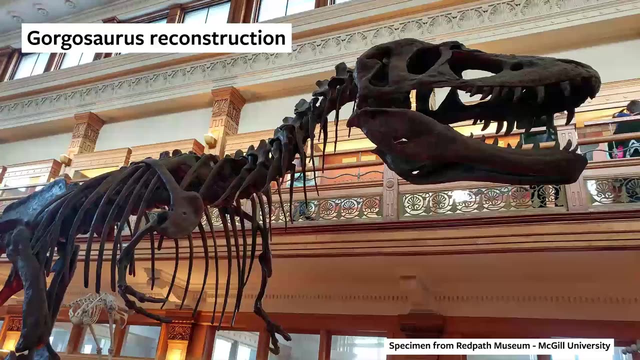 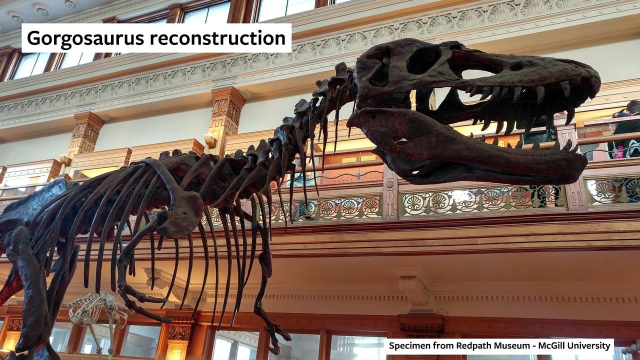 permineralized. This petrified wood became petrified when each of its microscopic cells were permineralized. just like the Brazilian agate, The same thing happened to the bones of this dinosaur. Not all fossils become permineralized, but those that do can then easily. 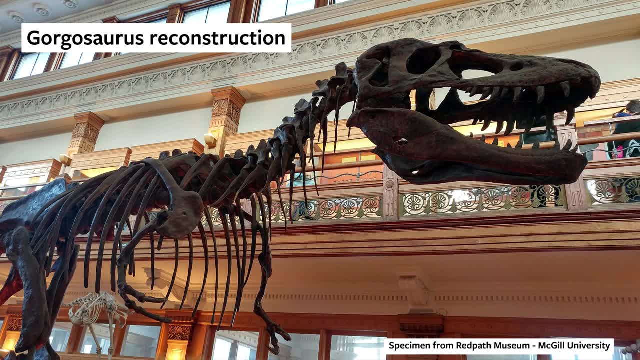 last for a long period of time. This is the case with the Brazilian agate. This is the case with the Asian agate. The Brazilian agate is known to survive for hundreds of millions of years, Any preserved body part, excrement or impression of an organism that lived in. 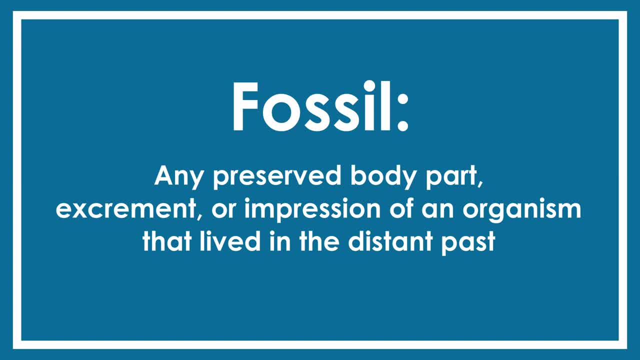 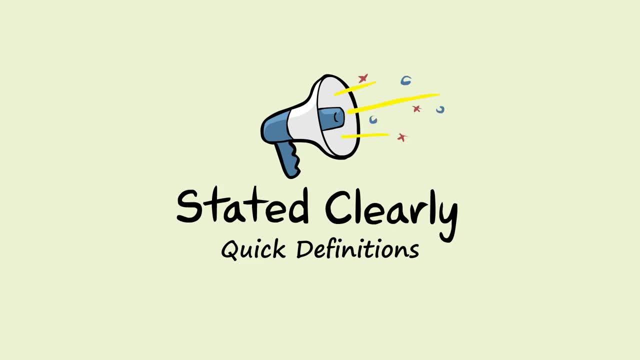 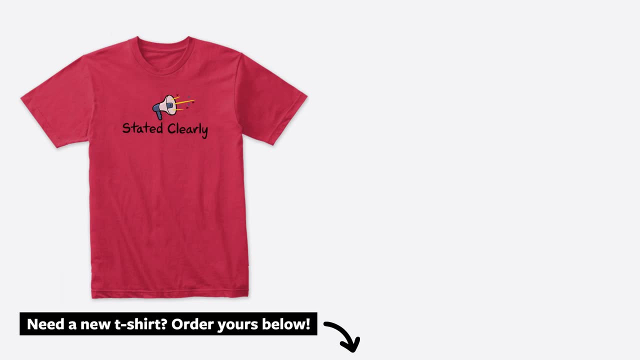 the distant past. I am John Perry and that was a quick definition of a fossil stated clearly. Thanks for watching. If you liked it, make sure to give a thumbs up and subscribe, because right now I am publishing new quick definitions every other Monday. 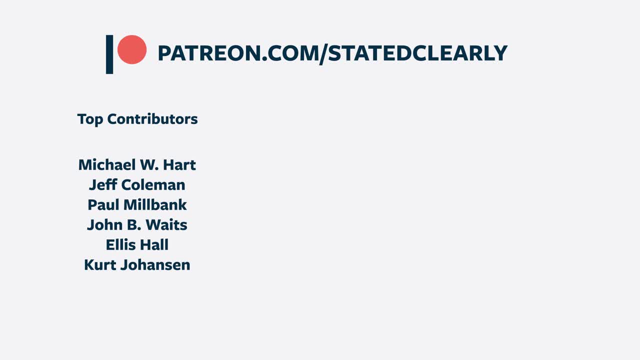 This video series is funded by good people like you who support me by contributing monthly to my efforts on patreoncom. forward slash stated clearly. If you'd like to help out, I'd appreciate it. So long for now, stay curious.